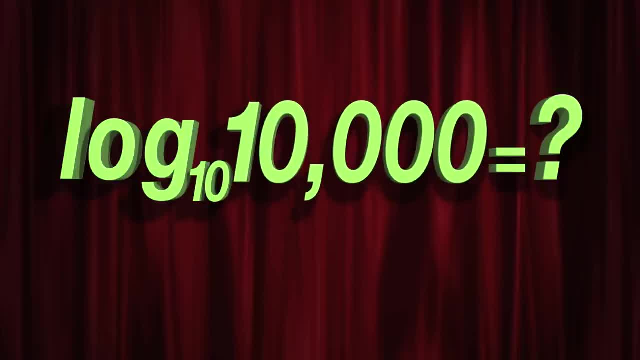 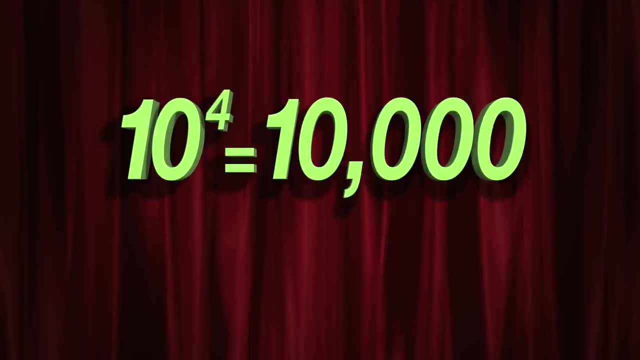 with an example: What is the value of log base 10 to 10,000?? The same question could be asked using exponents: 10 raised to what power is 10,000?? Well, 10 to the fourth is 10,000.. So log base 10 to 10,000 must equal 4.. This example can also be completed very. 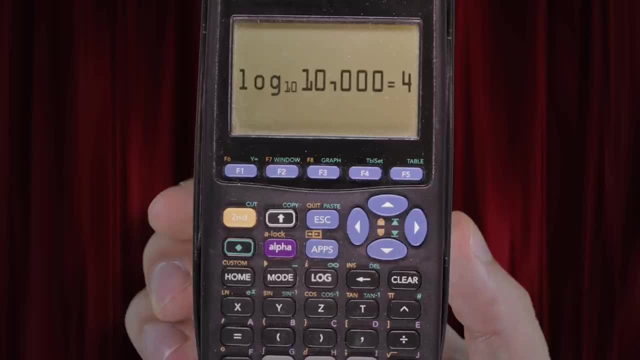 simply on a scientific calculator Log base, 10 is used so that it is equal to 10 to the power of 10 to the power of 10 to the power of 6.. This is the same formula used so frequently in the sciences that has. 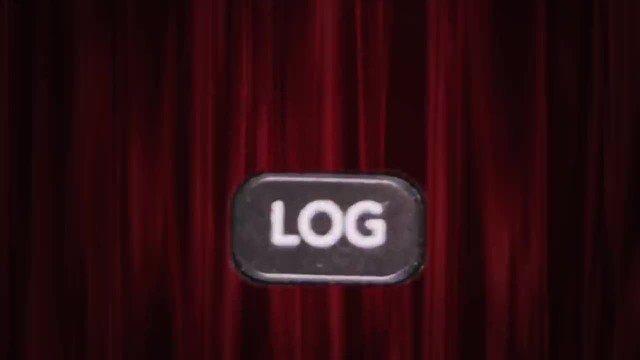 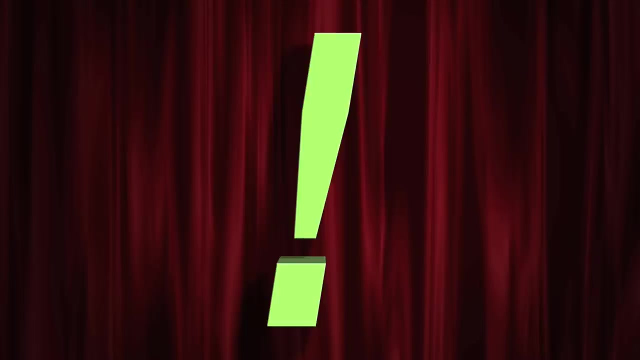 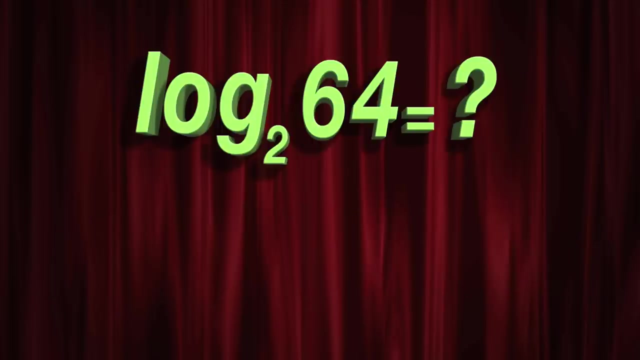 the honor of having its own button on most calculators. If the calculator will figure out logs for me, why study them? Just a quick reminder: the log button only computes logarithms of base 10.. What if you want to go into computer science and need to understand base 2?? So 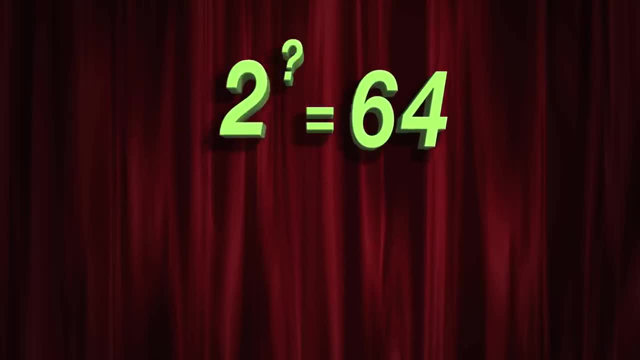 what is log base 2 of 64?? In other words, 2 raised to what power is 64?? Well, use your fingers 2,, 4,, 8,, 16,, 32, and up. What is log base 2 of 64?? Well, what is log base 2 of 64?? Well, use your fingers 2,. 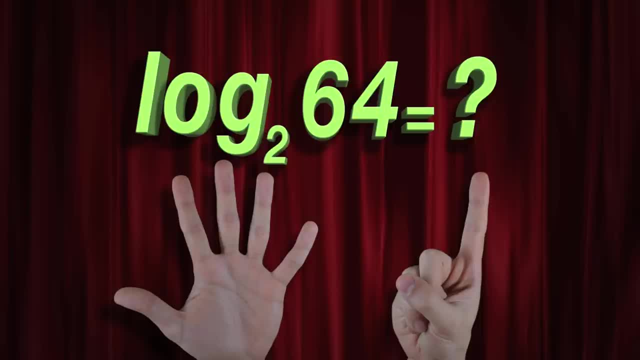 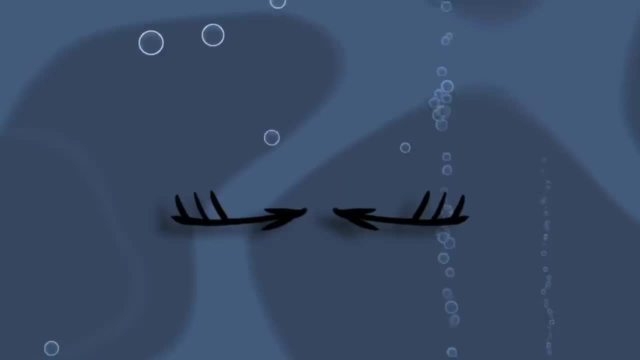 4,, 8,, 16,, 32, and up 64!. So log base 2 of 64 must equal 6.. So what does this have to do with my eyes turning red in some swimming pools and not others? 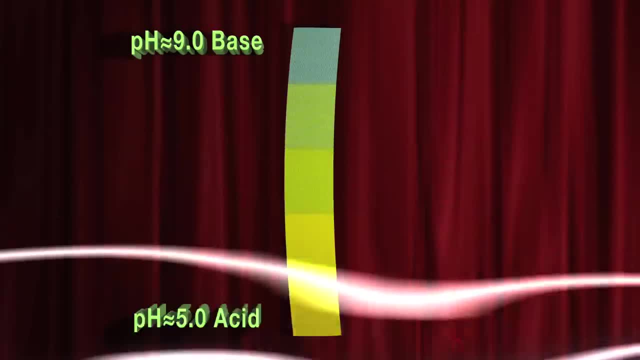 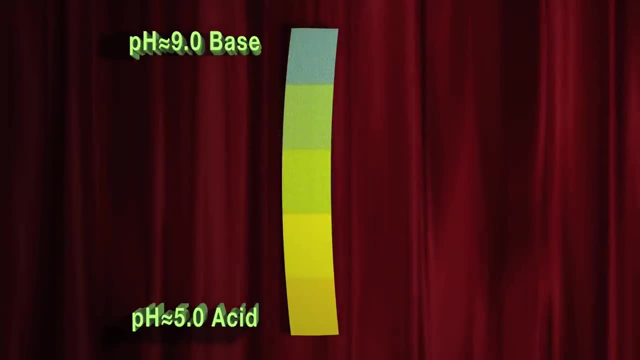 Well, it leads us into an interesting use of logarithms in chemistry: finding the pH of water samples. pH tells us how acidic or basic a sample is and can be calculated with the formula: pH equals negative log base 10 of the hydrogen ion concentration. 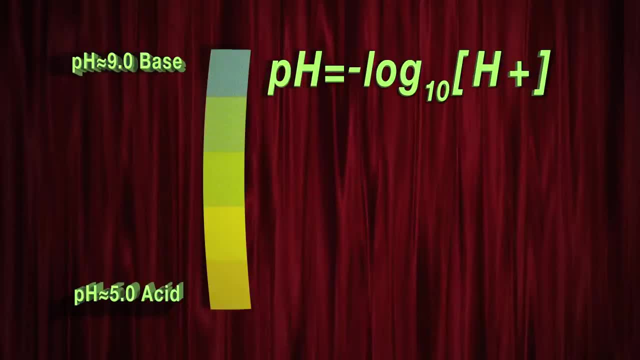 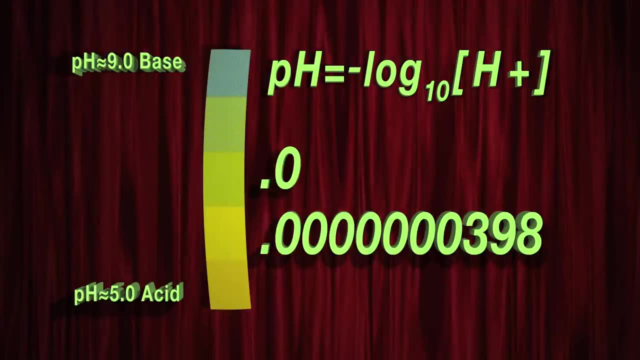 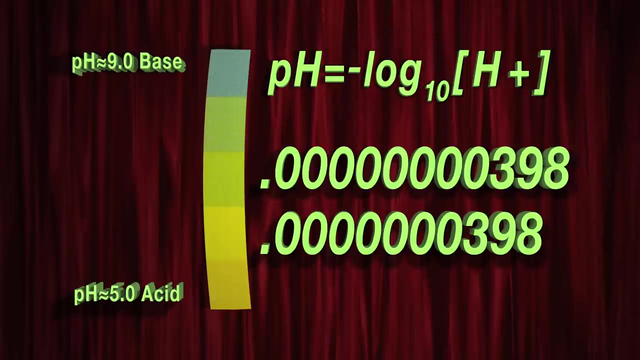 or H+. We can find the pH of water samples with hydrogen ion concentration of 0.00000000398 and 0.00000000398 quickly on a calculator. Punch negative log of each of those numbers and you'll see the pHs are 7.4. 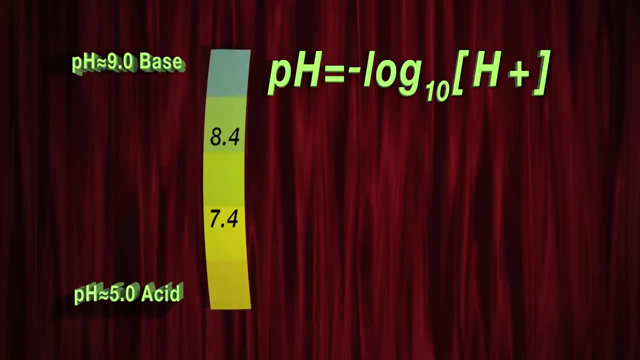 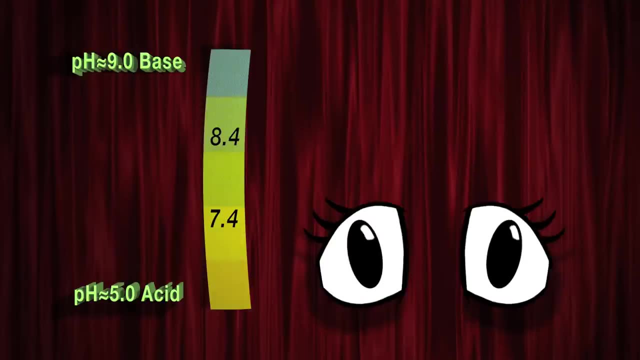 and 8.4.. Since the tears in our eyes have a pH of about 7.4, the H-plus concentration of 0.00000398 will feel nice on your eyes, but the pH of 8.4 will make you feel itchy and red. 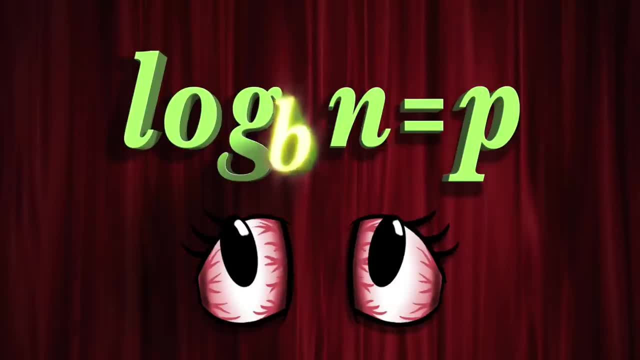 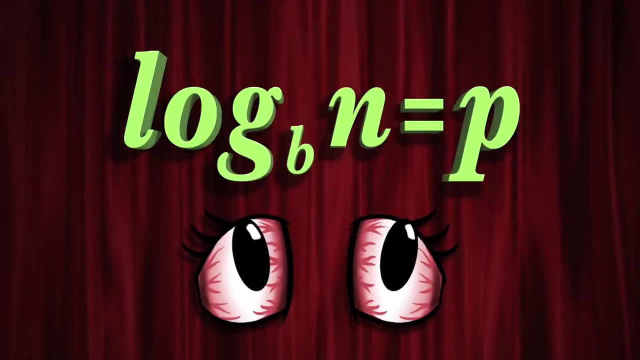 It's easy to remember logarithms: log base b of some number, n equals p, by repeating: the base raised to what power equals the number. The base raised to what power equals the number. The base raised to what power equals the number. So now we know logarithms.